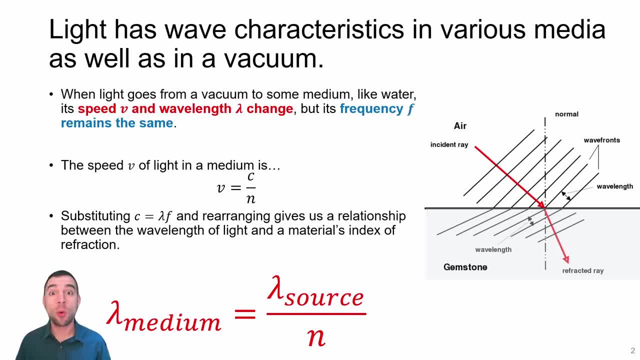 But in any other medium the index of refraction will cause for that light to slow down in the medium. We actually find that the wavelength of the light in the medium is what changes when its speed changes. The frequency of the wave is strictly set based on the source, that is. 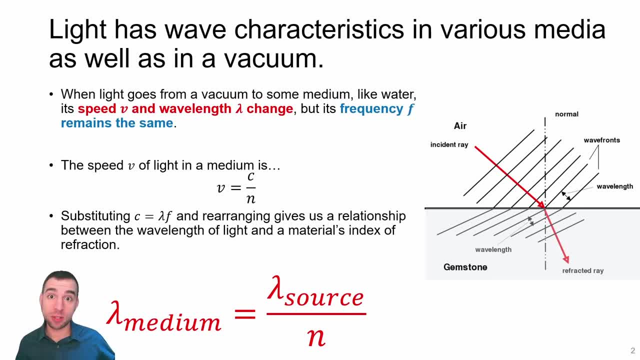 outputting those waves. So when a wave enters a new medium and slows down, its wavelength will correspondingly go down, And this means that the wavelength of light in a medium and the medium's index of refraction are related And we can use this equation in the bottom here to determine what the wavelength of light will be in a specific medium. 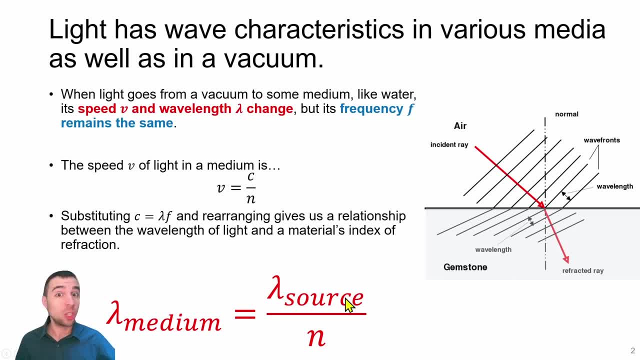 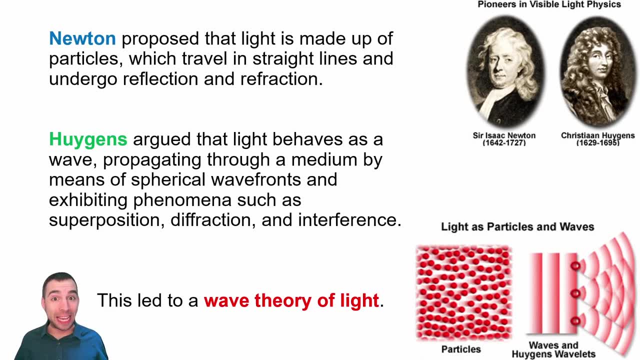 based on that medium's index of refraction And what the true wavelength of the light is being emitted from the source. This whole idea about light being a wave, when it was actually a very serious debate between Isaac Newton and Christian Huygens. Newton believed that light was a particle. 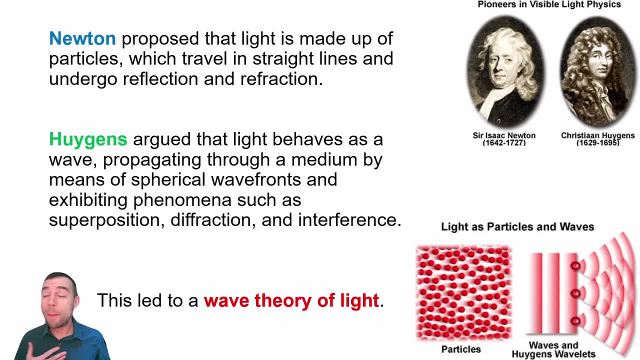 meaning that it traveled in a straight line and it could bump into things like the doorway or the windowsill and it would be blocked, creating a shadow. This understanding of light makes a lot of sense and it's very consistent with our macroscopic understanding of light. But Huygens. 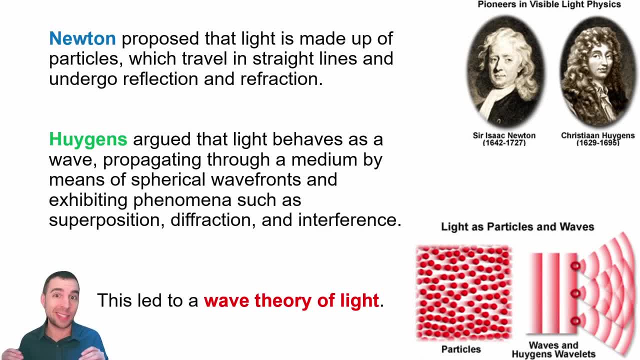 proposed that actually light was not made up of particles and instead light is a wave itself, And the only way that we could prove if light was a wave was if it obeyed laws and demonstrated phenomena that were characteristic of waves, like superposition, interference or diffraction. 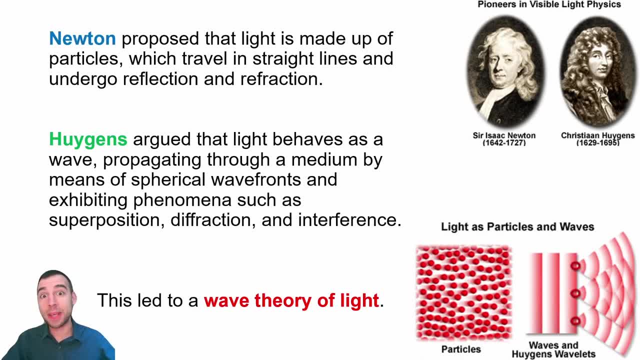 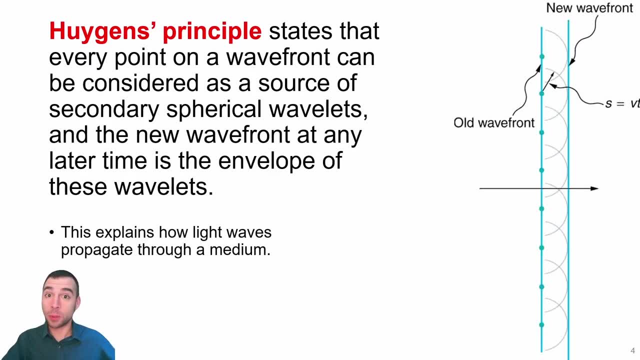 In the end, we find that light does behave as a wave, indeed, and we call this the wave theory of light. Huygens' principle is basically a way of understanding waves, which says that each point on a wave essentially acts like a source of another, smaller, 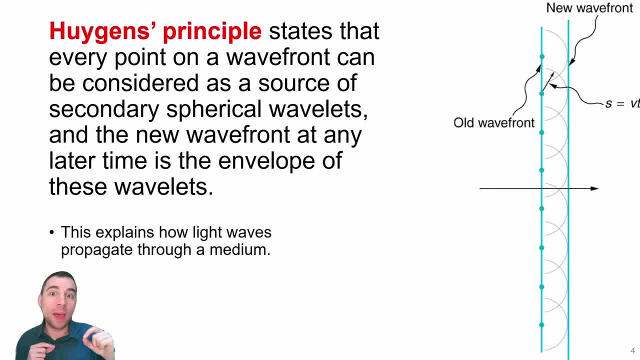 wavelet. If every single point on a wave creates its own little tiny spherical wavelet, we can see that those individual wavelets always add up to have their wavefront be at the edge of the wavelet, and this essentially describes how light travels. For example, if we sent a beam of light, 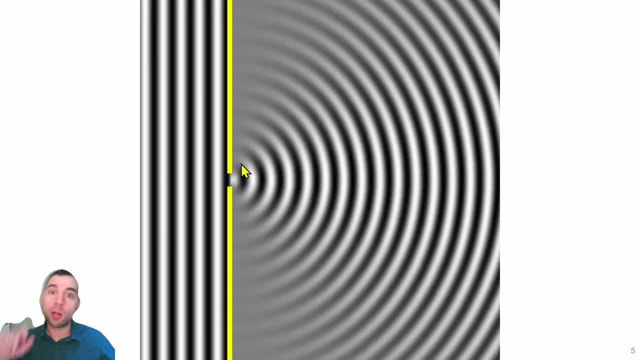 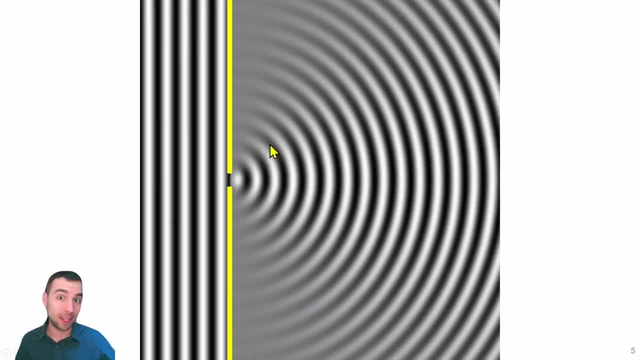 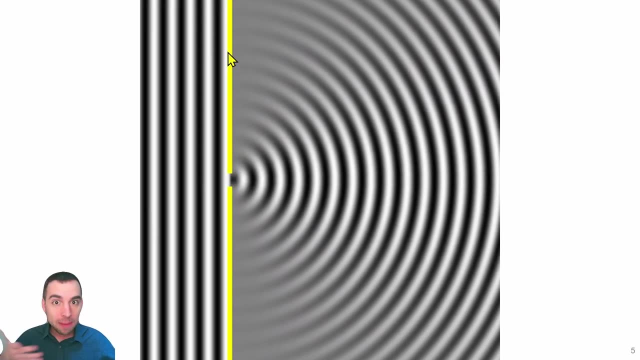 toward this small hole and we only let a small little bit of the light through, we would see that the light would spread out in a circular fashion. This is the wavelet coming from just this individual point, and if we had every single one of these points open, we would have many, many circular wavelets that would add. 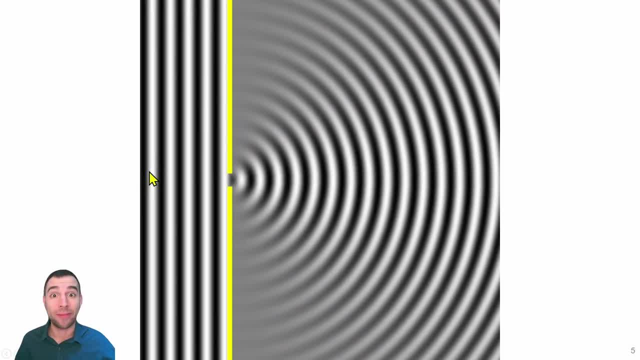 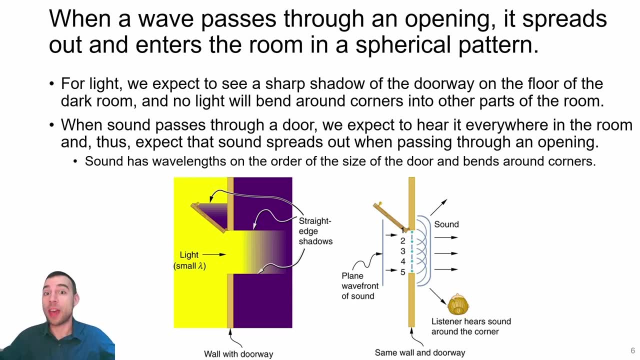 together to essentially create the wave fronts that you see on the left here. And as a wave enters through some kind of opening, it typically spreads out into that opening. But this is a little different between light and other waves. For example, with light, when we have a doorway that's open, the light will only 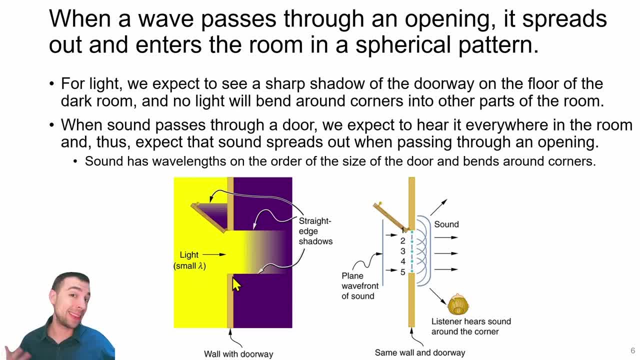 enter where the doorway opening is, and then it will not spread out and fill the room. there will still be a shadow specifically where the light does not hit. Now, this is different for other waves like sound. If you have an open doorway and a sound wave is entering through that doorway, it's not like there's a shadow of sound anywhere. 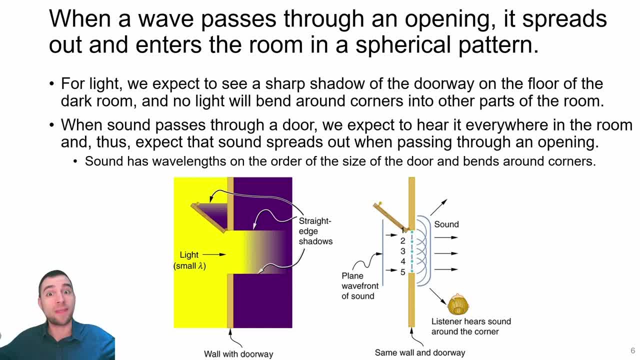 the sound spreads out and enters the entire room and fills it. The reason this happens is because sound has wavelengths that are much closer to the actual length of the opening itself. so if we can shrink down a doorway opening to be just a very small slit, so we can only let a small 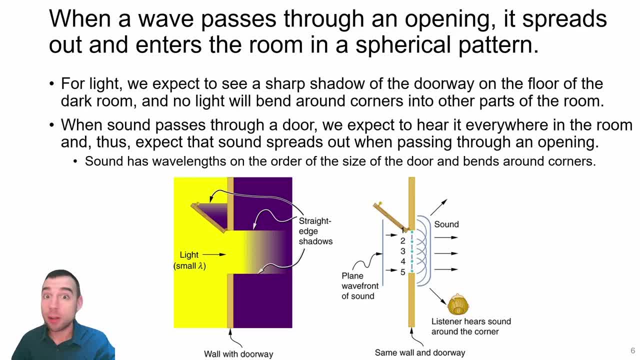 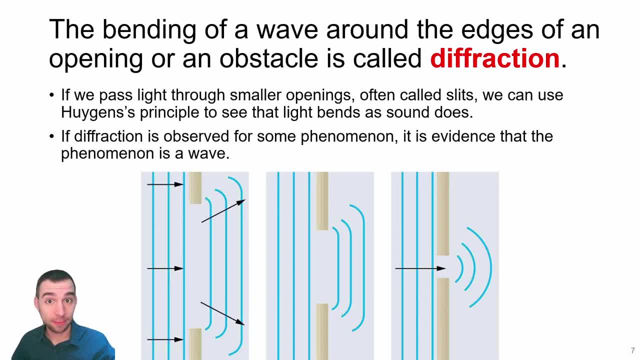 amount of light waves through, then we will see that light waves also do this bending. The bending of a wave around an edge or obstacle is called diffraction, and if that opening gets smaller and smaller and smaller, the effects of diffraction are more and more severe. 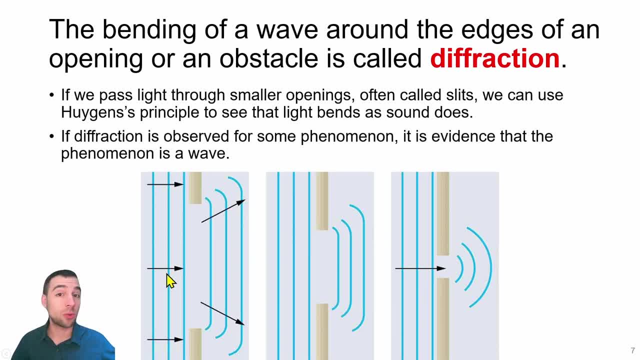 and more noticeable On the left. here we have light waves entering through a doorway and we can see that there's a small amount of bending here, and as the opening gets smaller, the degree of bending, the diffraction becomes more significant, until we have a very small opening and now the light waves bend and 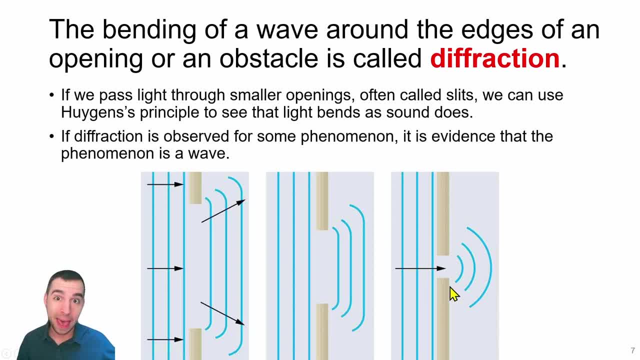 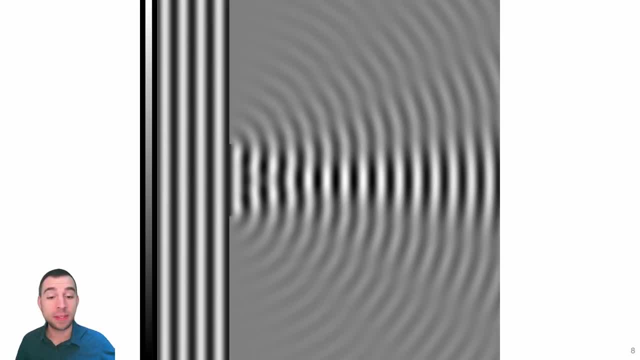 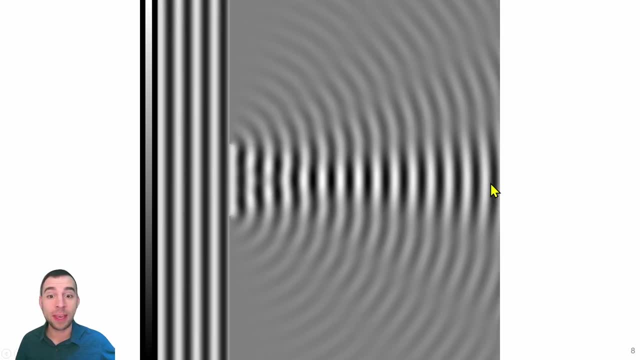 create these circular shapes rather than a straight path, like you would have seen before. that would have created a shadow. For example, here you can see light waves filling a room. There's a slight bend on the two edges, but mostly in the path where the light is traveling, It just travels in a straight line and lets 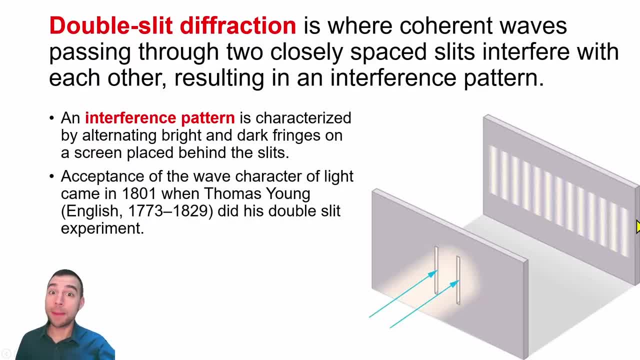 light travel there. There are several major types of diffraction, and the most common one is called double slit diffraction. Double slit diffraction occurs when we let light pass through two very small holes in the middle of the path. This is called double slit diffraction. 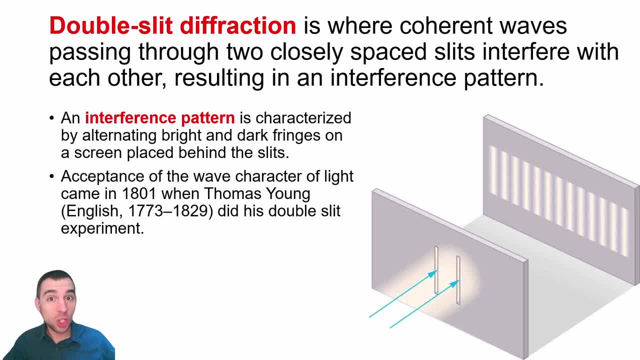 Double slit diffraction occurs when we let light pass through two very small, narrow slits and you might expect for the shadow on the opposite end of these two slits to just have two vertical lines, sort of like the shape of the opening that the light is traveling through. but actually we get something. 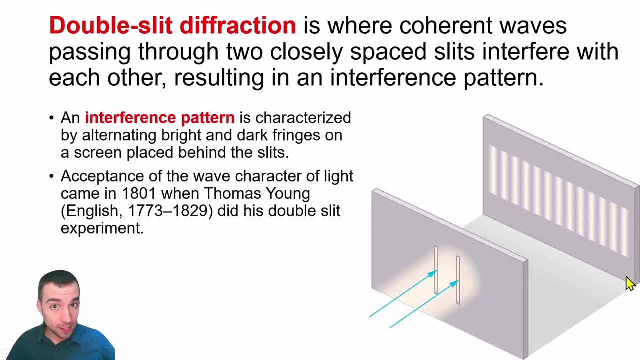 different. We get several vertical lines all lined up together. We call this an interference pattern. There are bright spots and dark spots that the light creates at the top and bottom of the slits as it passes through those openings and as it experiences diffraction. This experiment was basically what proved that light is. 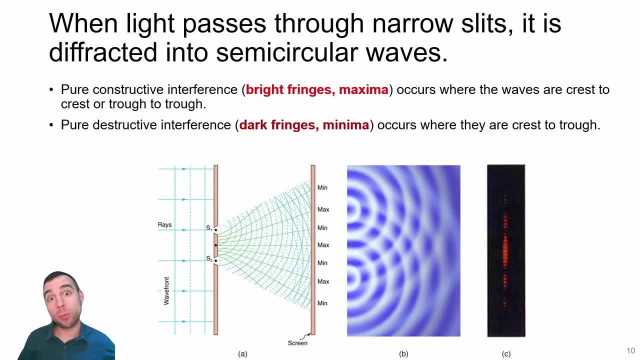 indeed a wave. As the light waves travel through both of those two different slits, each slit acts like its own source of small light wavelets that will travel out in a circle, And so if the top and bottom slits each let, circles out you. 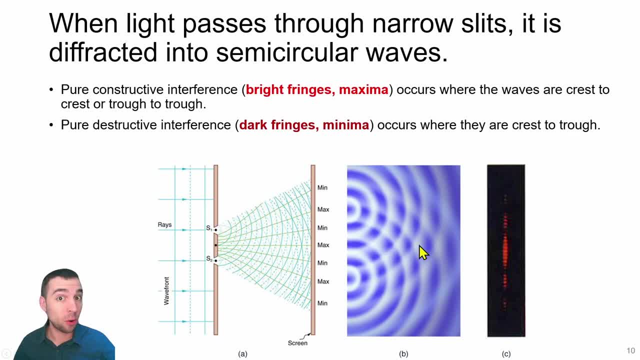 will see that there are points where the two circles overlap. they're wave-like and they overlap. There are points where wave fronts are perfectly aligned, leading to constructive interference, and then there are other spots where the wave fronts are anti-aligned, experiencing destructive interference As these two slits let 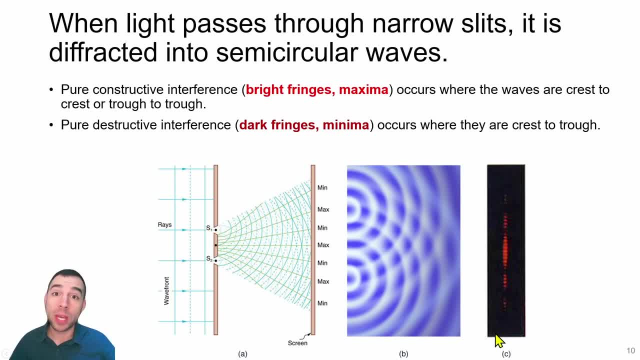 light through, we will create an interference pattern that looks sort of like what you see here. Here we have a red laser being shined through only two slits, but it creates these many lines that have bright spots and dark spots. The bright spots are where there's perfect constructive interference. we call those. 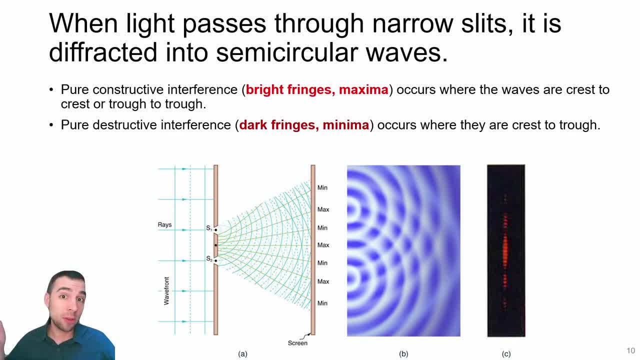 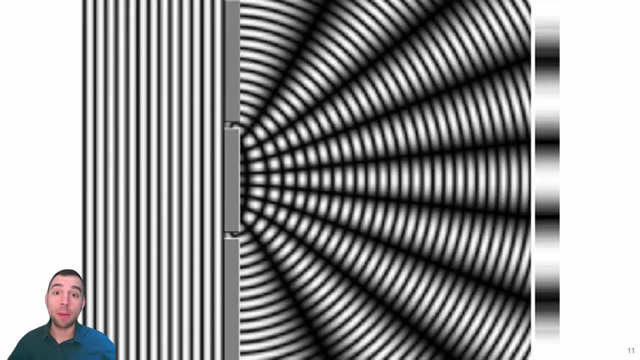 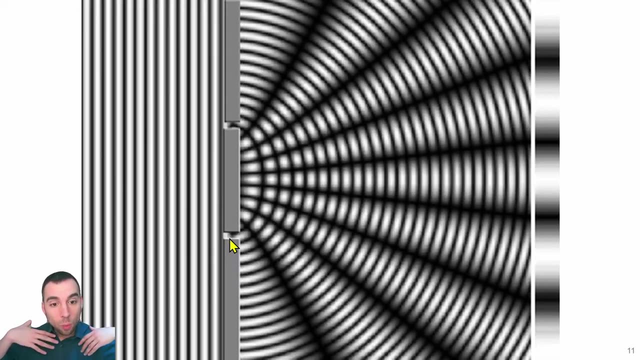 bright fringes or maxima, and the dark spots are where there's perfect destructive interference. we call those dark fringes or minima. So here you can sort of see an example of double slit diffraction. We have our laser light coming in, we have our two openings here and the way that the wavelets travel. 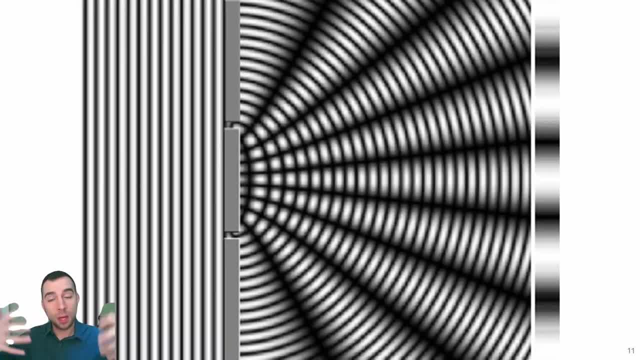 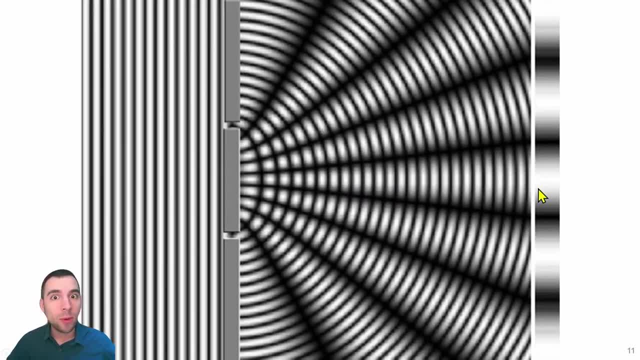 out. just because there are two different sources, each with circular wavelets traveling from them, we get this pattern. here We're along this line. we have a very bright spot with wavelets adding together with constructive interference, and then right next to that, we have a little line. 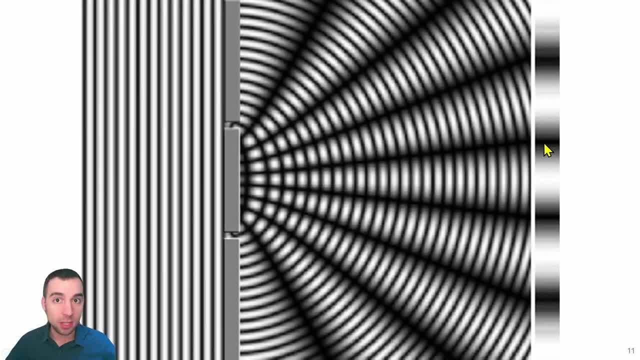 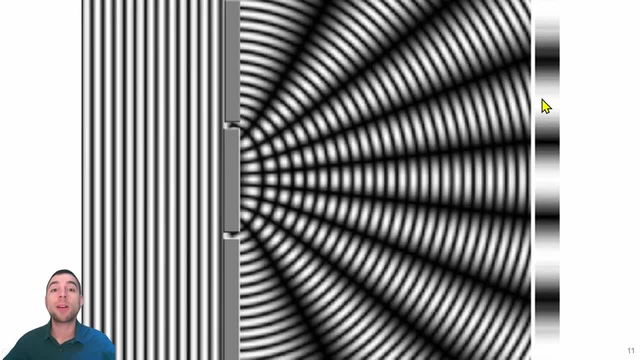 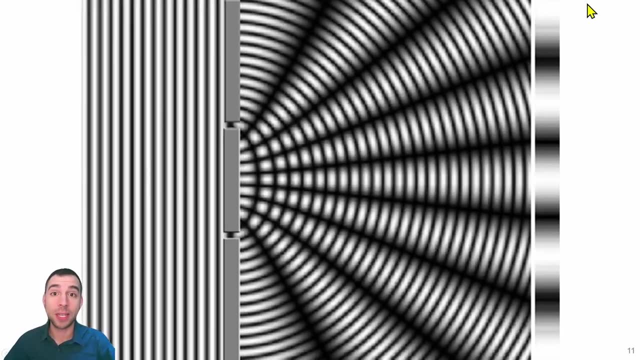 that is a dark shadow where we have perfect destructive interference and the waves do not add together, they cancel each other out, And then the next bright spot occurs, and then another dark spot, and then another bright spot, and so on, and that interference pattern will happen for a double slit diffraction. 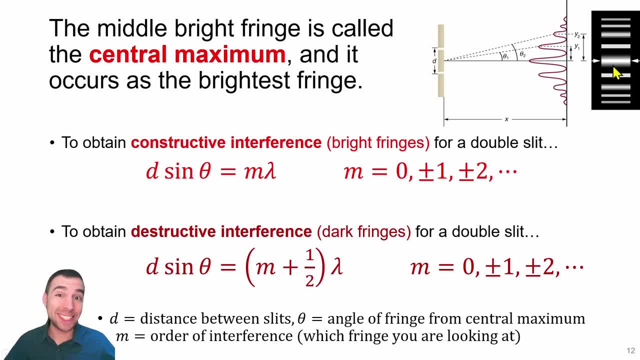 situation. We call this a double slit diffraction. We have a center bright spot, the central maximum, and this will always be the brightest, it'll have the most intensity and then any spot beyond that. we call the next fringe either a bright fringe or a dark fringe. We can calculate where. 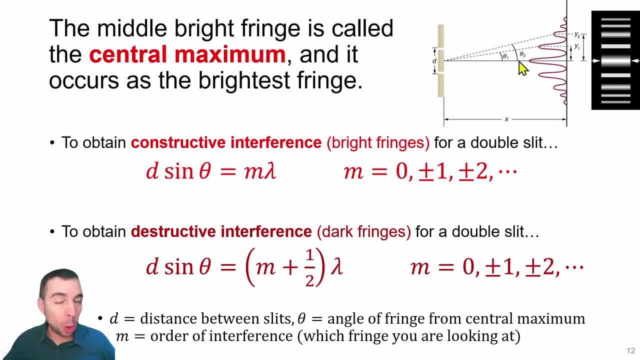 our bright fringes will occur, at what angle they will be deflected from the central maximum. using this diffraction equation d sine theta equals m lambda, If you can plug in integer values or zero for this m number, depending on the wavelength of your light. 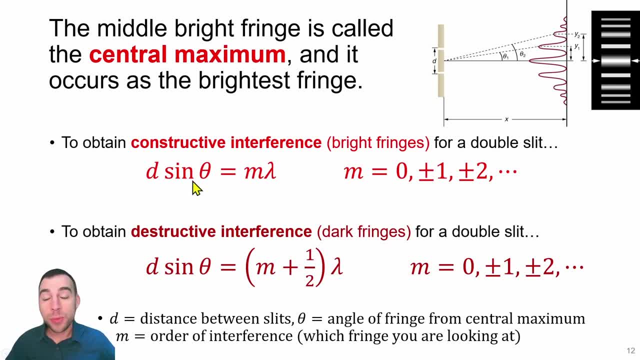 that you're shining through and the distance between your slits, you can predict what angle each bright fringe will be deflected at. We can do the same thing for dark fringes with destructive interference. The only difference is that we add a little 1 half to that integer. 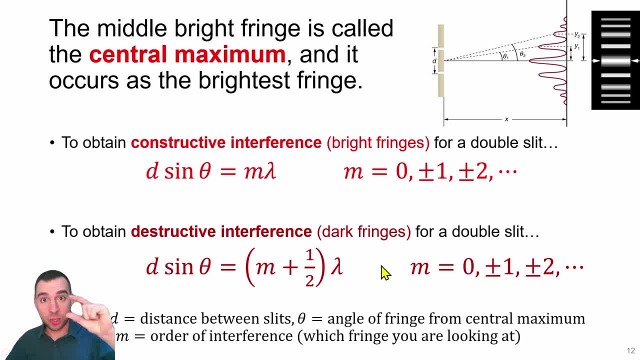 m value. So again, d is the distance between the two slits, theta is the Deflection angle from the central maximum. an M we call the order of interference. It will tell you which bright fringe or dark fringe you are at. The central peak has an M of 0.. 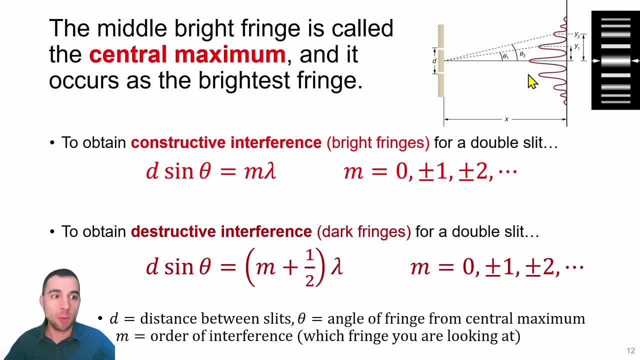 And then if you go one above the central maximum or one below the central maximum, that will correspond to an M equals positive 1 or an M equals negative 1, depending on which way you go. And then, as we go out to farther bright fringes, we step up in our order of interference number. 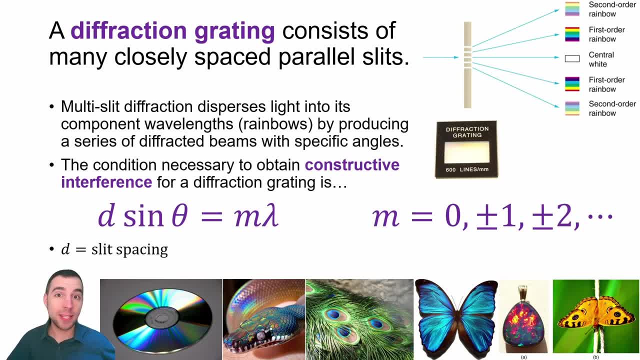 Another type of diffraction other than two-slit diffraction is called multi-slit diffraction, where we can use something called a diffraction grating that has many, many slits in it. If we shine light through a diffraction grating, we will see that it gives an interference pattern. 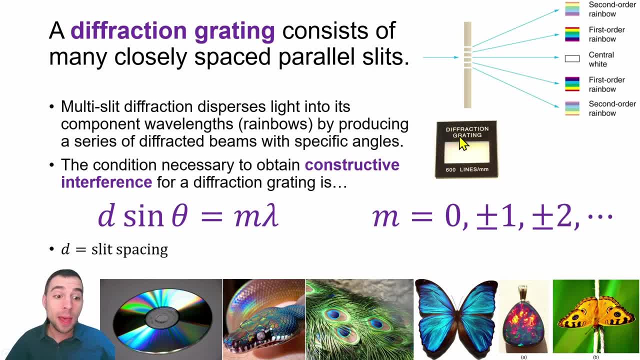 You can see a diffraction grating right here and you'll notice that it's not a diffraction grating. It is often given the number of lines per millimeter of the diffraction grating, And so if you invert this, you can figure out what the spacing is per line for some diffraction grating.